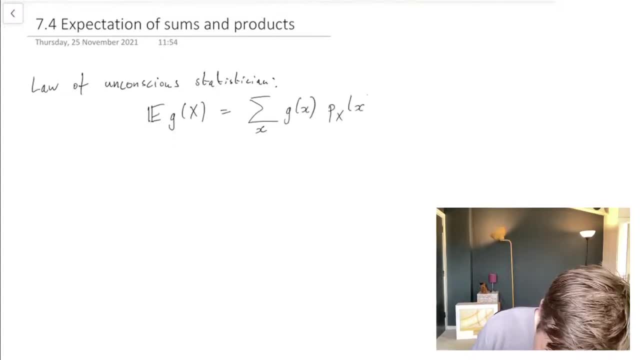 function of that x and you multiply by the probability mass function. So our new result here is what, if we want the expectation of a function of two random variables, like x plus y or x times y or some more complicated function of the two, And the answer is it's. 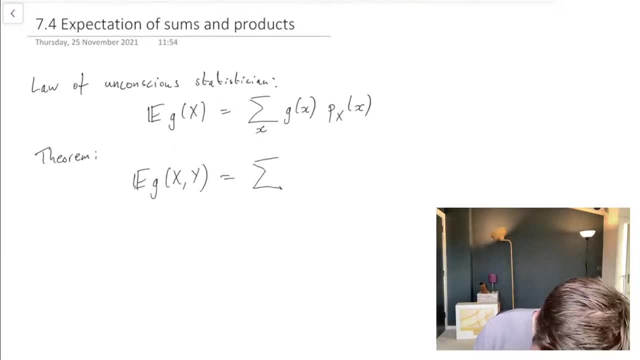 kind of the same. We have a sum which, instead of being just over x, is now over both x and y. Then we have the function, but it's not just a function of x now, it's both a function of x and y. And instead of just having a marginal distribution, px, we now have the. 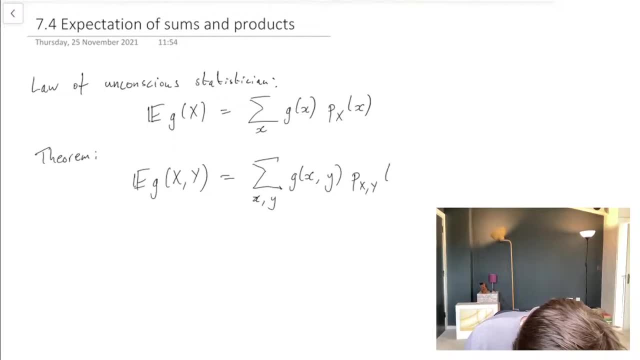 joint distribution pxy. So that's very similar to the law of the unconscious statistician. before. Two particularly important special cases is: what about the sum, the expectation of x plus y? Well, that turns out to be the expectation of x plus the expectation of y. Importantly, this is: 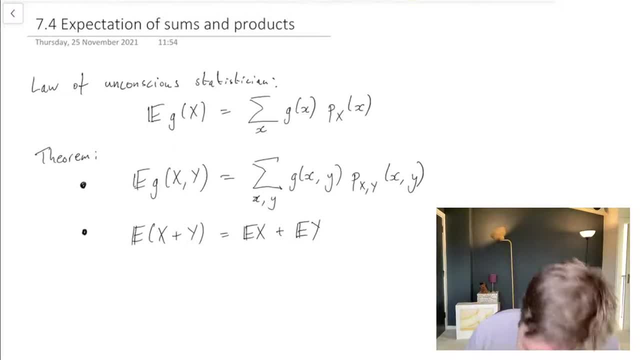 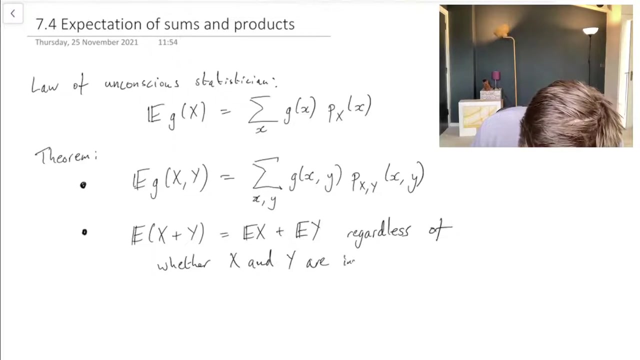 always, always true. So, in particular, it's always true. It doesn't matter whether or not x or y are independent. This is always true, regardless of whether x and y are independent or not. And we also might want to look at the expectation of a product. 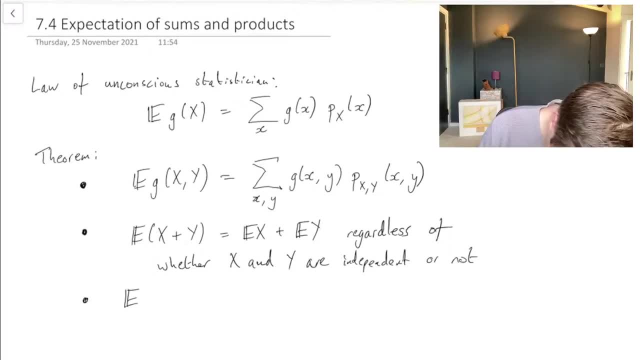 Yeah, that's right. Yeah, Yeah, Yeah. So that's not really true. That's not really true. that's not really true. expectation of x times y. Now, this does depend on whether they're independent or not. Turns out that the expectation of a product is the product of an expectation if 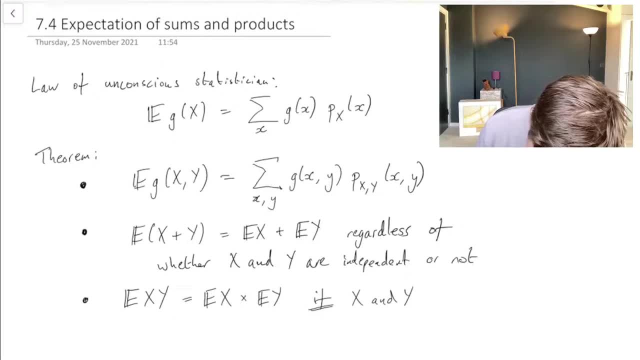 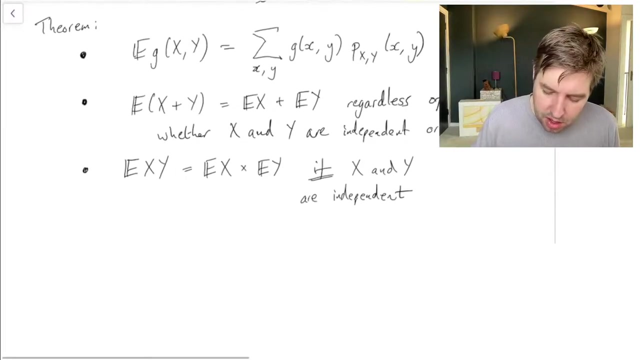 x and y are independent, So it's important to get this straight. The expectation of a sum is the sum of an expectation all the time, always. The expectation of a product is the product of an expectation if they are independent. If we combine this second result here together with previous results, we had about single random. 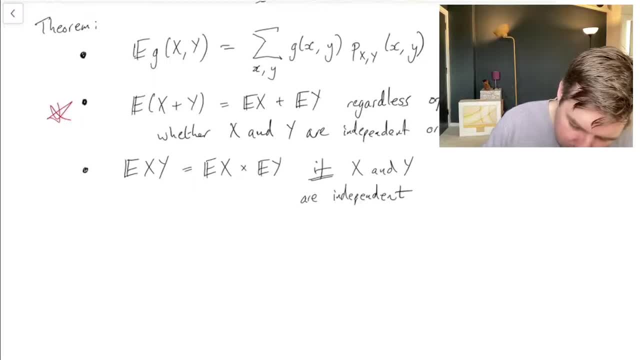 variables. we can kind of stick all those together, because with single random variables we looked at what happens if you multiply them by a constant. Here we looked at what if you add two random variables together and we also looked at what happens if you add a constant. 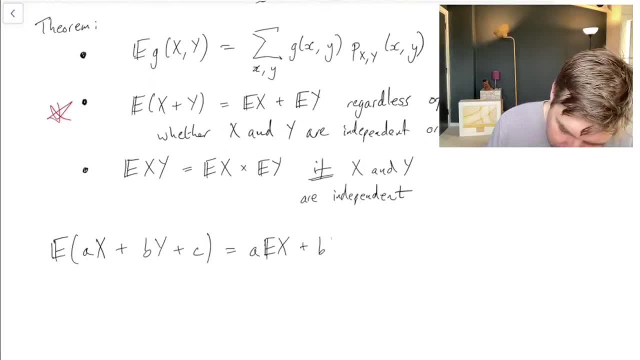 So you can see, by putting all those together we get this right. All the constants can come outside. We can split everything up separately. All works out neatly Like this. it's sometimes called linearity of expectation. Those of you who've been studying about vector spaces and things like that- 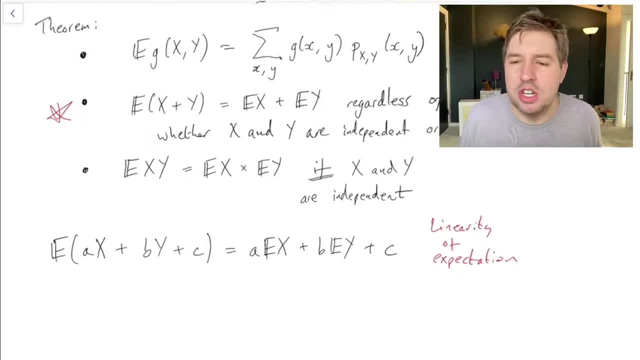 might recognize this as being basically the same thing as the definition of a linear map when you're talking about vectors. So the three bullet points in that theorem up above- I was hiding a bit with my face- those three bullet points. there are proofs of those in the notes. 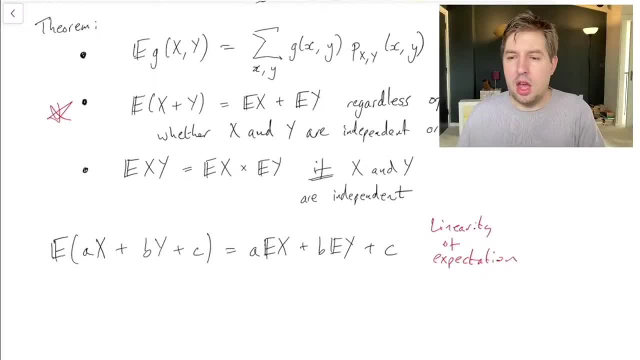 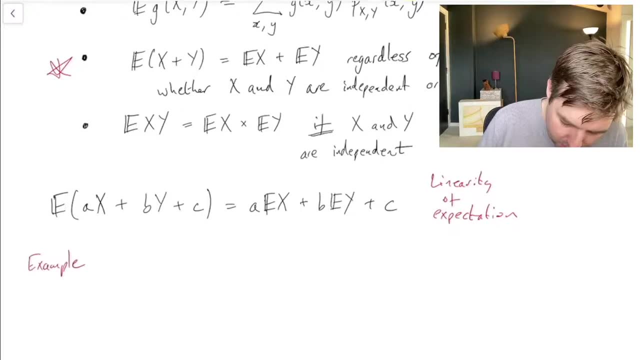 If you want to look at proofs, we will just do a quick example of how to use them, But in the next section, when we talk about covariance, we'll actually use these results a lot. So if you want more examples, skipping forward to the next subsection, 7.5,. 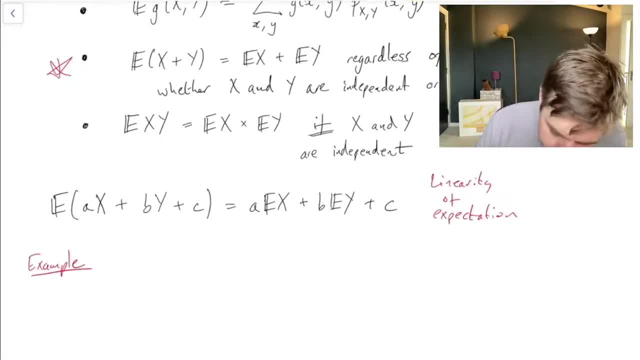 we'll give you more of those. But students answering questions on a problem sheet sort of forgets to write what the answer was. So this is a problem sheet. So this is. this is one problem sheet. We can do some more and we can do more of the others. 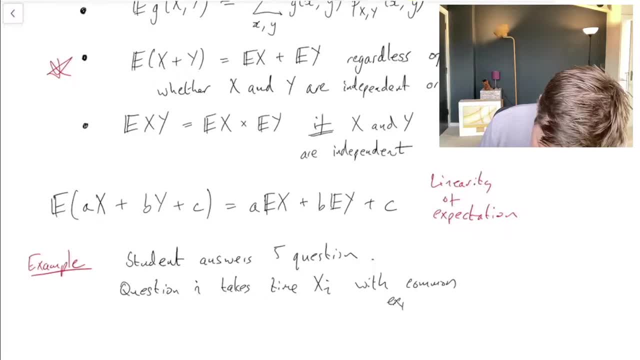 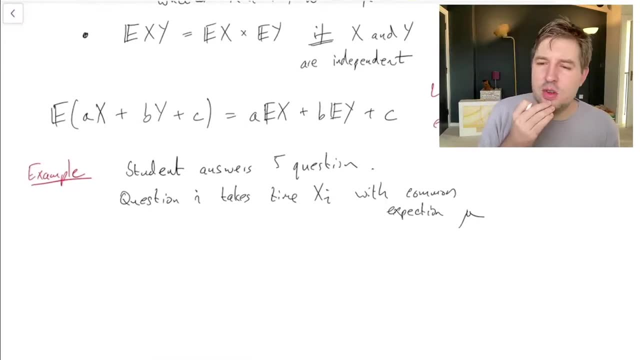 And here I'm gonna do the problem sheet, And each question takes a random amount of time with a common expectation, As in, they all have the same expectation, mu. So what's the total length of time it takes the student to solve all five questions on the problem sheet? Well, that's the answer I've just given you, But it's just that this problem sheet is a little far apart from the one we just showed you, And the problem sheet is just a value. So it's a quantity. It's the time we're going to use over time. 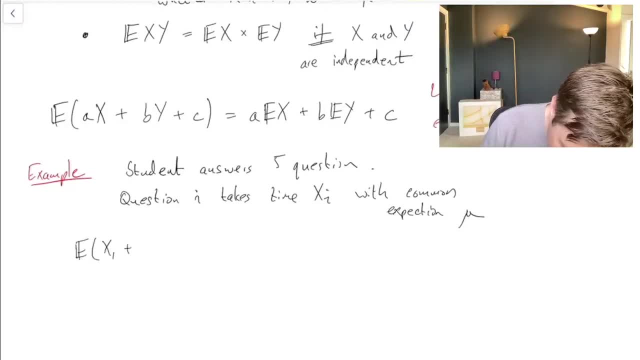 Well, that's the expected value of x1 plus x2 plus x3, plus x4 plus x5, but by this linearity of expectation result, this is equal to the expected value of x1 plus the expected value of x2, etc. so we can split up all the expectations and we get 5- lots of mu.